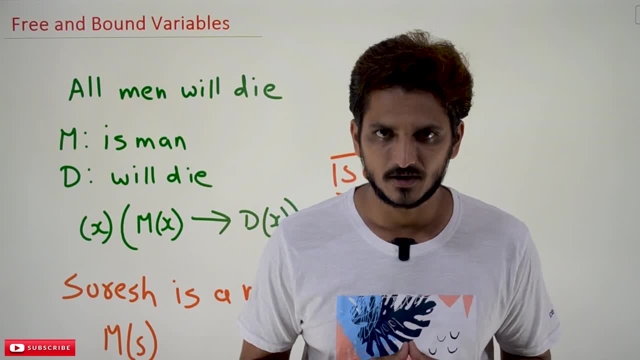 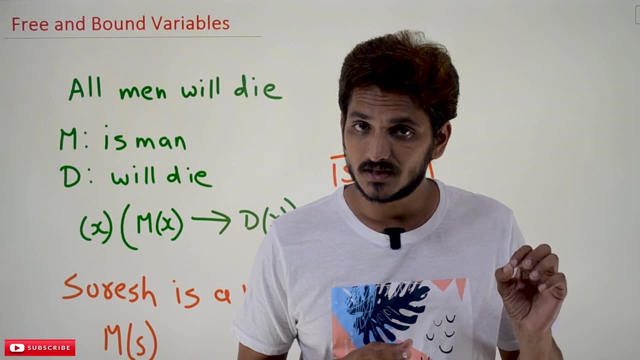 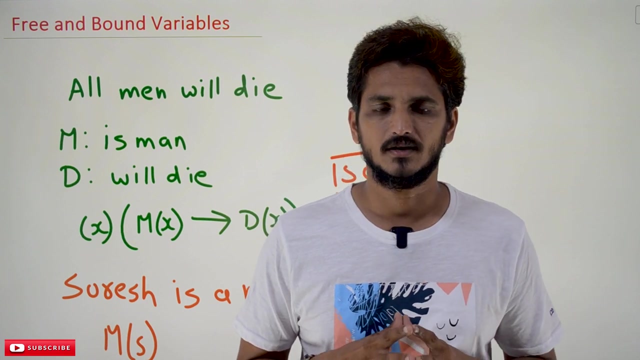 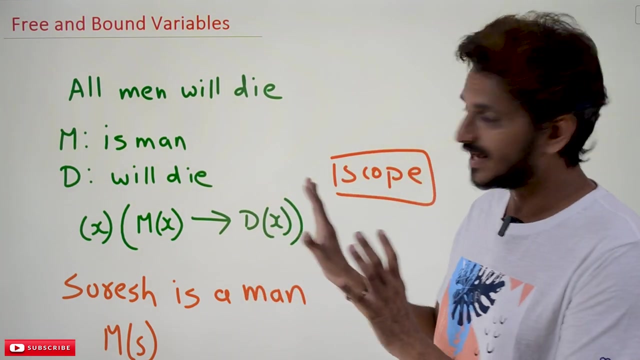 Hi, welcome to learning monkey. I am Raghu here. In this class we will discuss about free and bound variable. So in our previous classes we clearly discussed about this: universal and existential quantifiers. Please watch that class and come back here. The link for the playlist is provided in the description below. Coming to today's class, It's very, very easy to understand. We take an example and understand what's free and bound variable means. Let's take an example: all men. 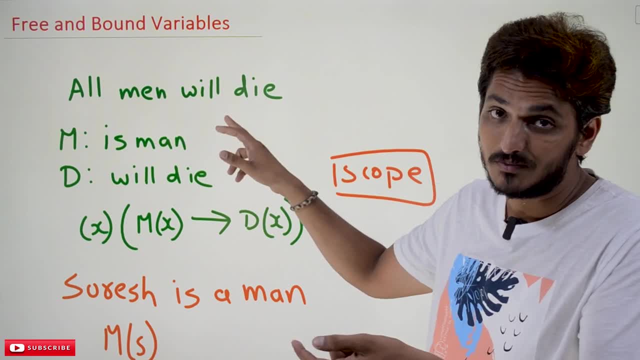 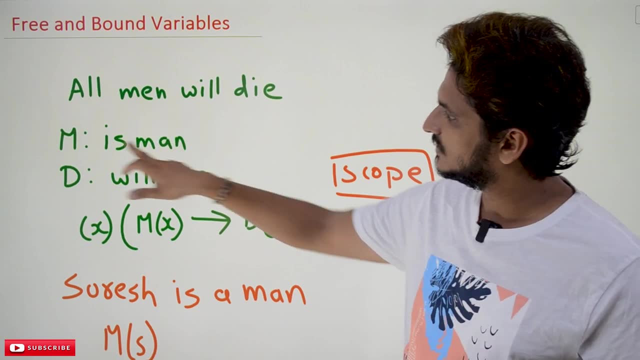 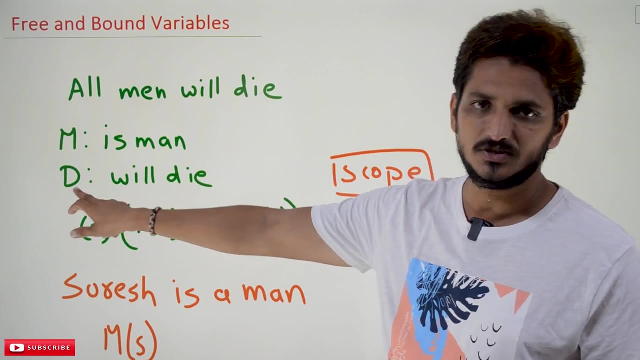 will die. So how we are going to write this statement in predicate function. These discussions made previously, So in this we are having two predicates: M is a predicate, It is called as a. is man Will die is a predicate, We named it as D. So how we are going to write this statement. 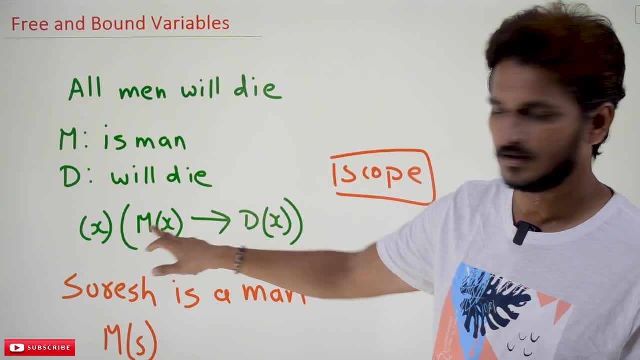 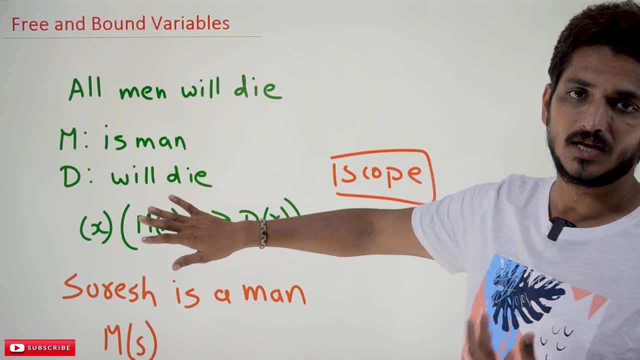 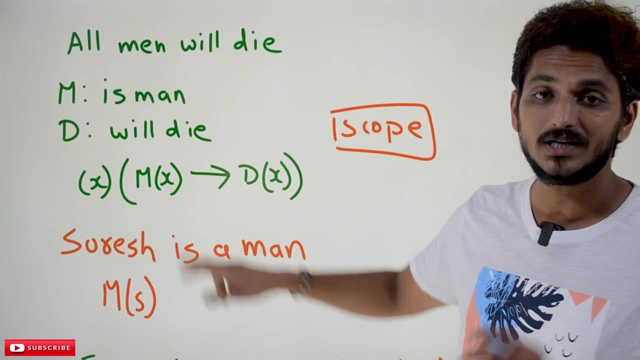 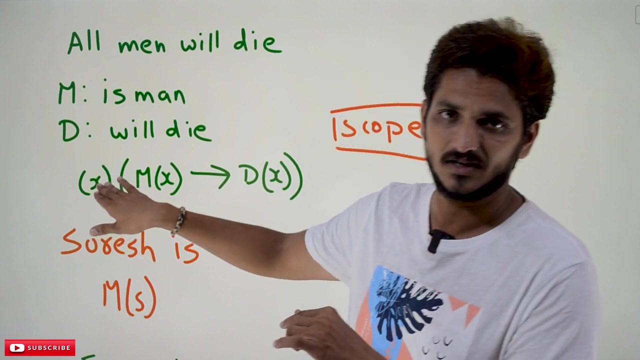 for all X. If X is a man, then he is going to die. X is going to die. This is how we write this statement in predicate logic. So in this, in this equation, in this equation X, we call it as bounded variable, because X is a variable that is bounded to the predicate, for all Means the point. 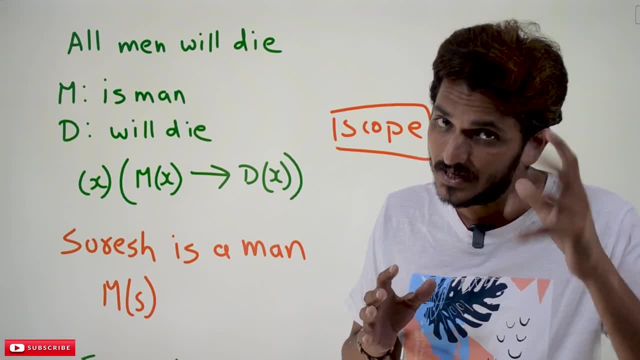 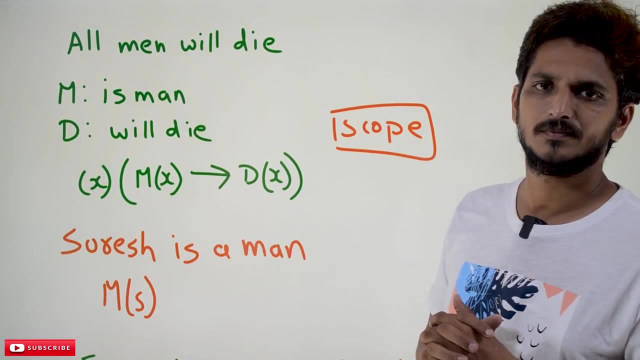 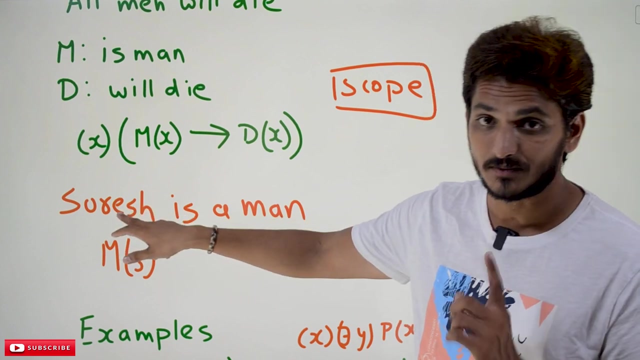 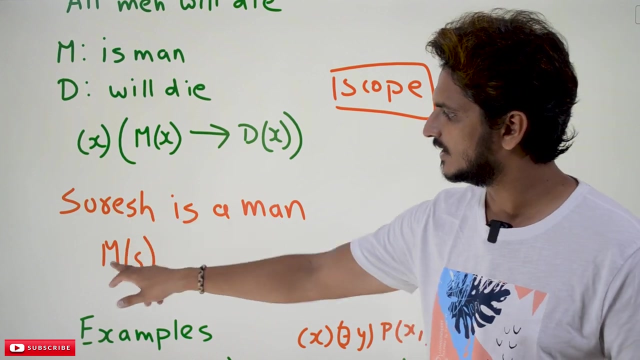 you need to understand variables that are bounded by any quantifiers. We call it as bounded variables. So take one more example. Suresh is a man, So Suresh is the subject. We will give a variable name to the Suresh subject. We named it as yes. This statement can be written as M of yes. 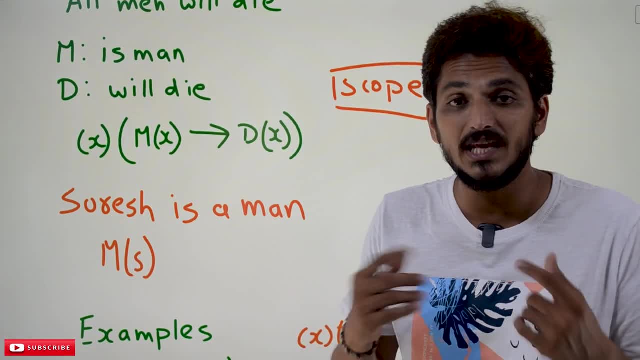 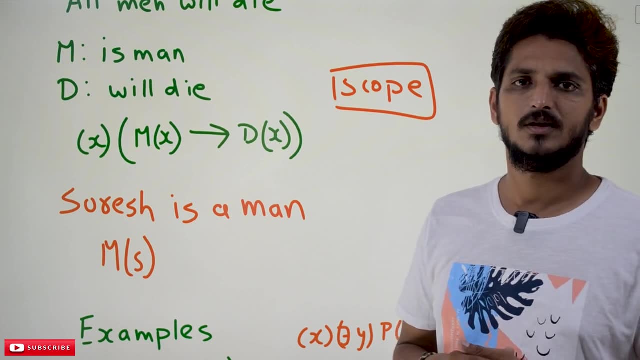 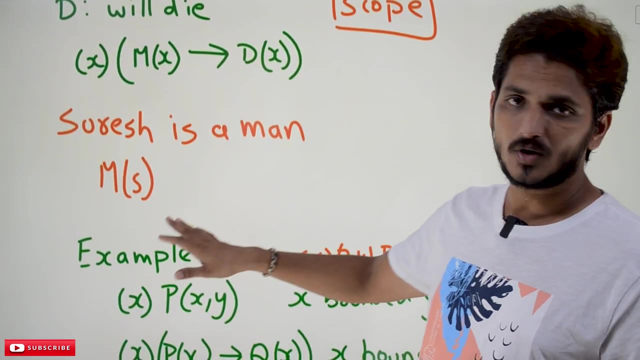 Here S is a variable which is not bounded by any of the quantifier. These type of variables we call it as free variables. So variables that are not bounded by any of the quantifiers, we call it as free variables. And one more important point you need to understand here: Suresh is a subject We 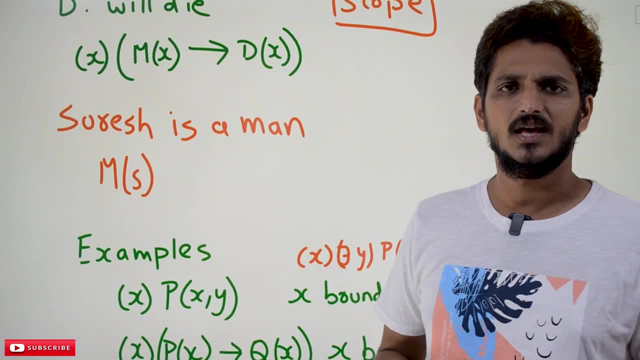 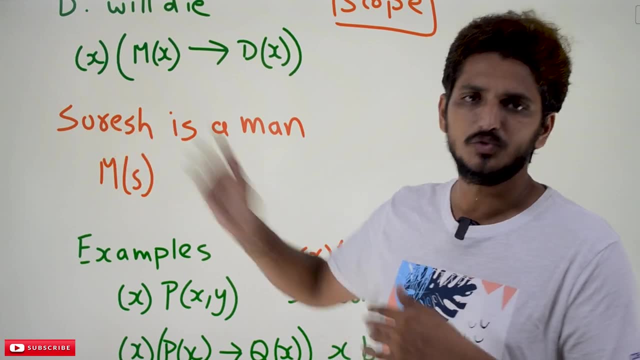 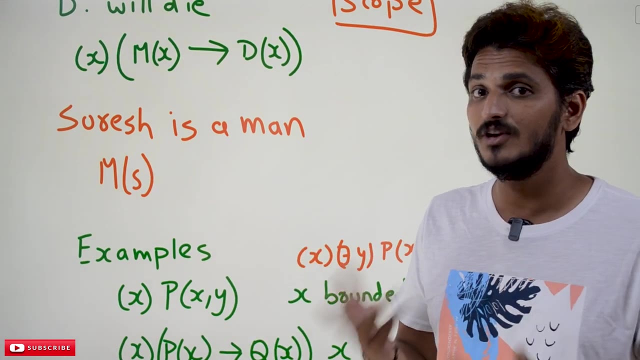 named that subject as a variable name. called yes, So you can give any of the variable name, not only a some. some of them they are going to give you variable name you as Suresh. Some of them- they are going to give H as a variable name for Suresh. You can give any variable name that is not a. 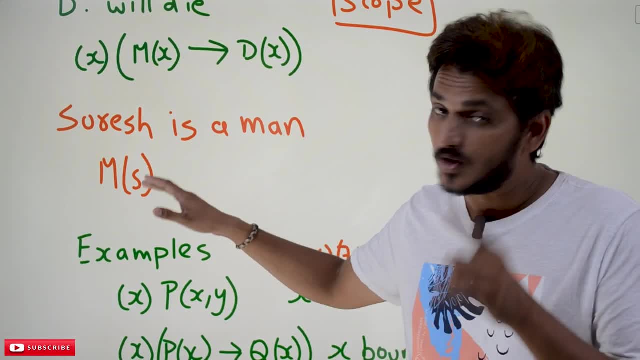 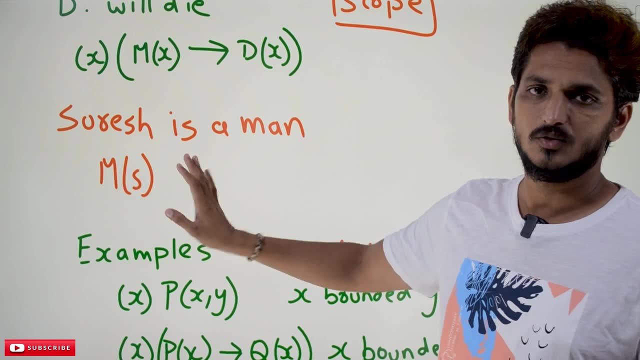 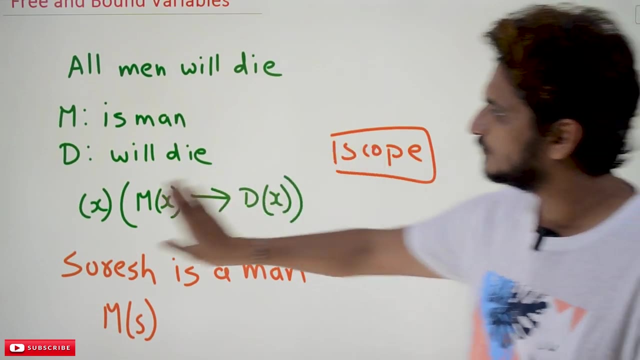 problem. So why we are going to say this is a this point we are going to use in our coming classes. By changing the variable, it is not going to affect anything. You can give any of the variable name for a subject. And one more important point: you need to understand what is the scope of this. 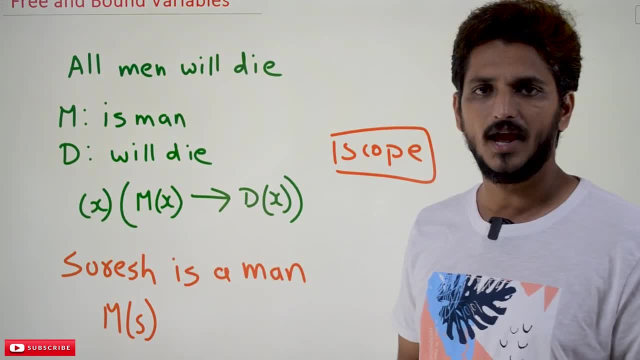 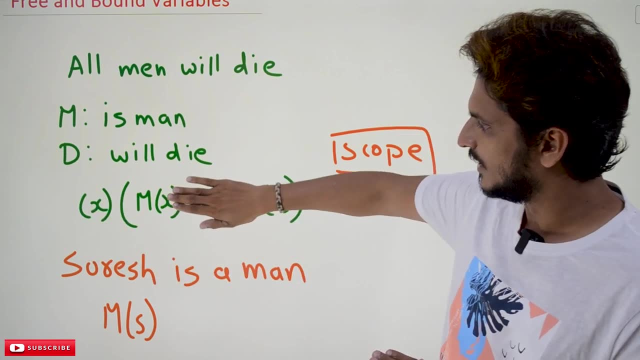 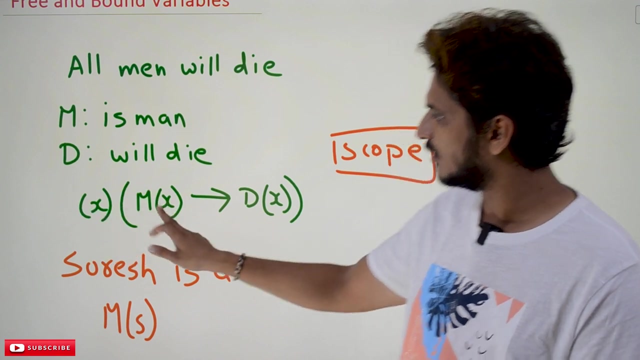 variable X. This quantifier for all X, The scope of the variable is: whatever the statement, This is the statement. So, before this statement, this quantifier has been mentioned. So the scope of this quantifier belongs to the subject. So the scope of this quantifier belongs to the subject. 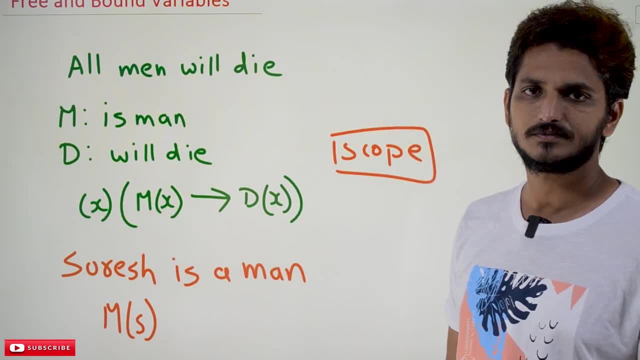 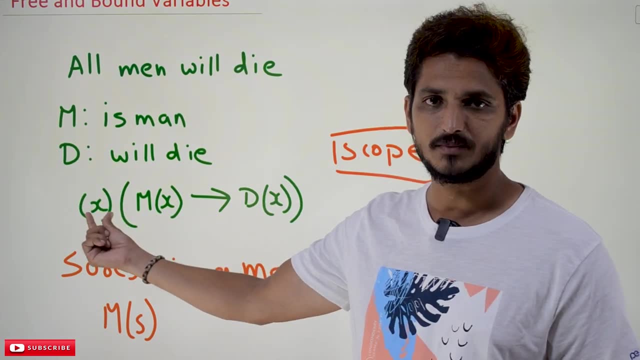 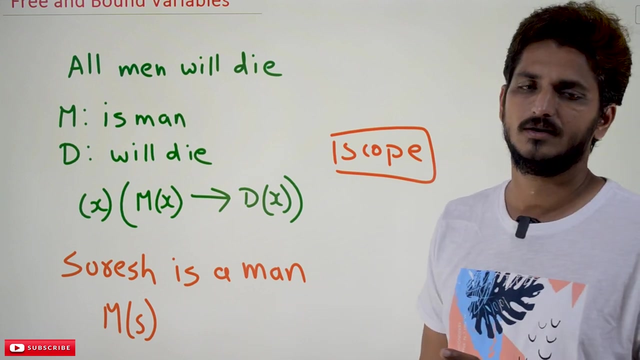 So the scope of this quantifier belongs to the statements, To this entire statement. See, you need to observe the brackets carefully. Brackets, brackets. before this we applied the quantifier Means this quantifier is applied to this entire equation. That is what the scope of the quantifier 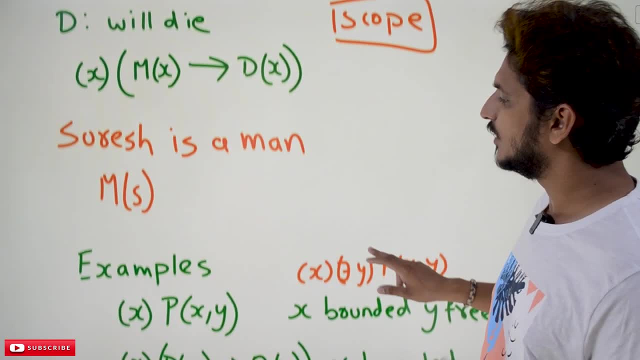 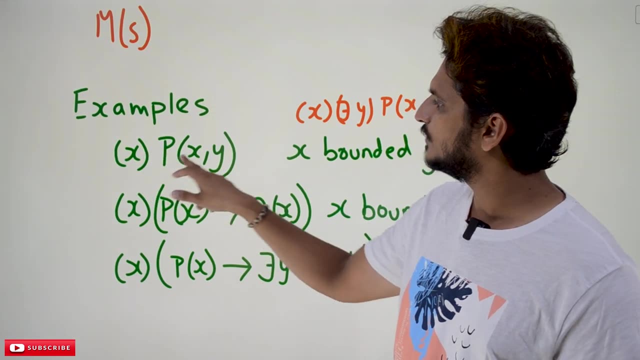 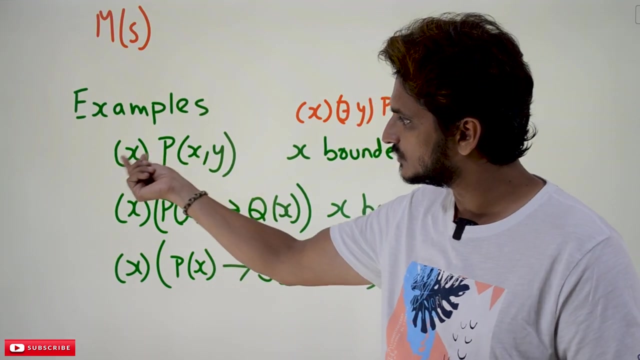 The scope of the quantifier belongs to this equation. Now we will take some examples and understand what is free variable and what is bounded variable. Let's take this example, for all XP, of yes, x, comma, y, So our quantifier, place it before the statement. So this quantifier, the scope of this. 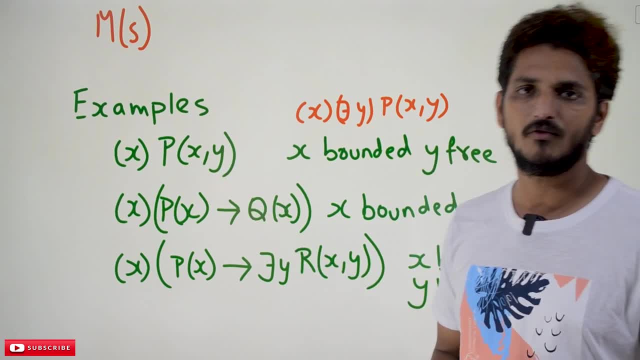 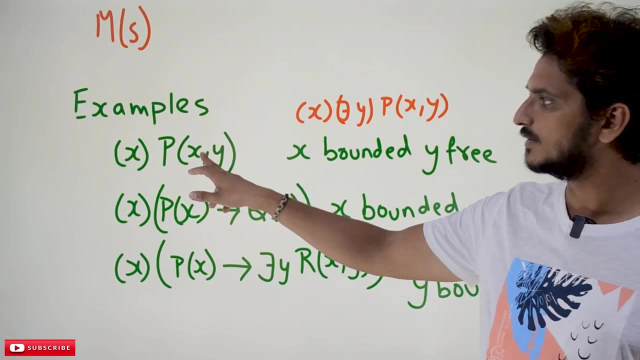 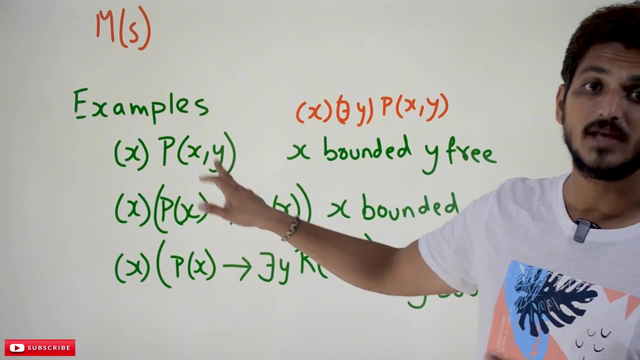 quantifier belongs to the statement p of x comma y. So in this x is a bounded variable or free variable. x is a bounded variable because it belongs to a quantifier, It is bounded by a quantifier. So x is a bounded variable, y is a free variable. x is a bounded variable, y is a. 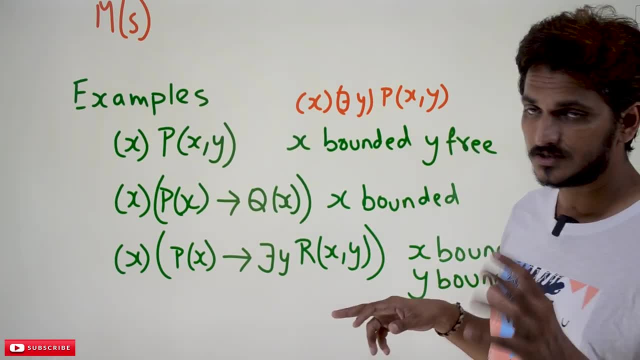 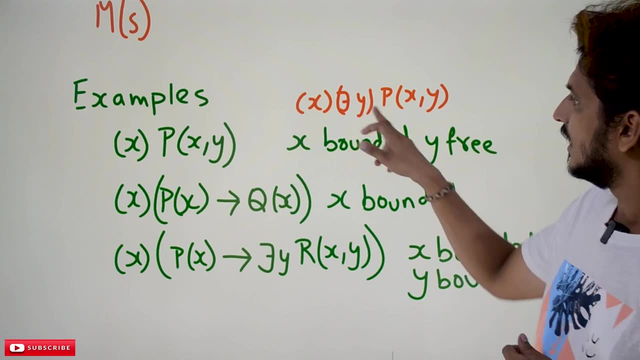 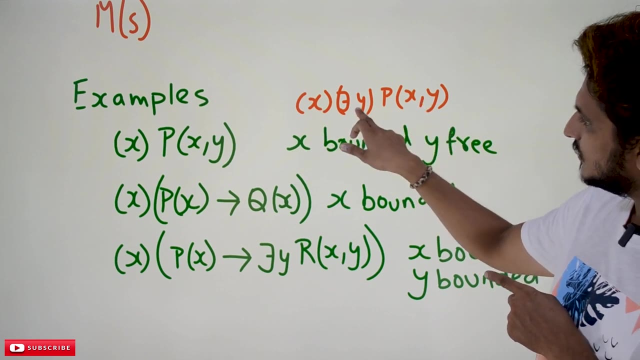 free variable. Let us take one more example for better understanding of that. For all x there exists y, p of x, comma y. So what is the meaning of that? This quantifier belongs to. this means the scope of this quantifier belongs to this equation. The scope of this quantifier belongs 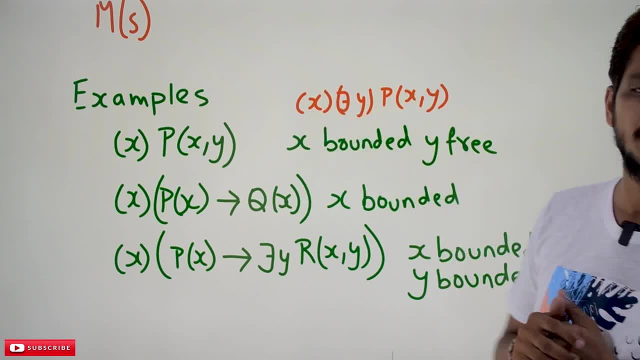 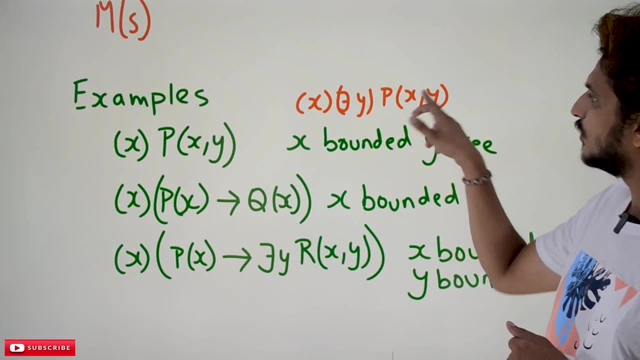 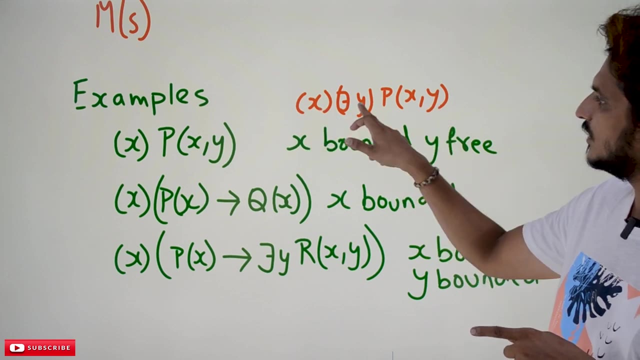 to this equation because before this equation, these quantifiers has been mentioned. For all x there exists y, p of x comma y. So now, in this situation, both x and y are bounded variables, because the x is bounded to this quantifier, Y is bounded to this quantifier.